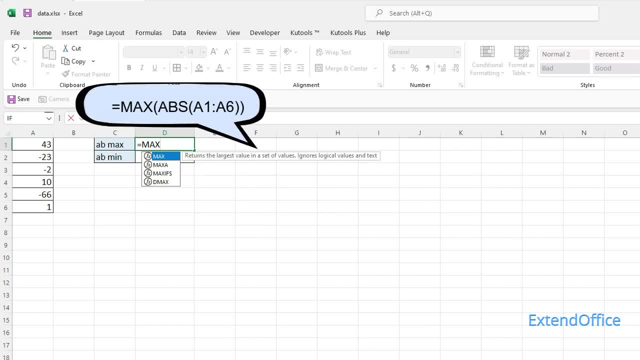 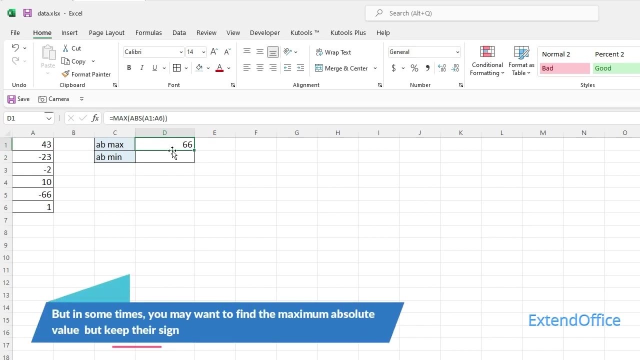 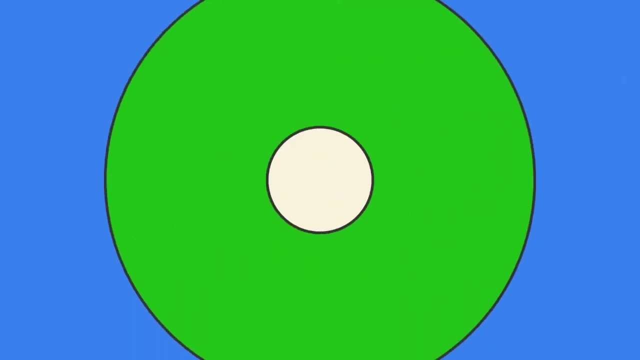 But in some times you may want to find the maximum absolute value but keep their sign. Here this video introduces the formulas that can find and return the absolute max or mean value from a range and keep the sign. Find max or mean absolute value and keep sign. 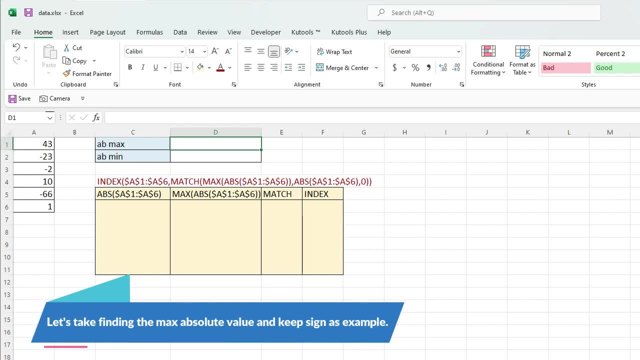 Let's take finding the max absolute value and keep sign as example. The formula that can solve this job combines several functions. here I divide it into four parts to explain it better for you. First, using abs function to list all absolute values of the values. 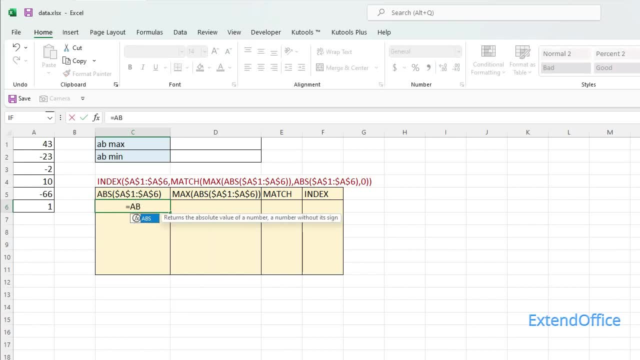 The first is the array function and in some old Excel versions you need to press shift and enter keys together to get all results. Then go to the array function and find the maximum absolute value. In the following two examples I have chosen the maximum absolute value and keep the sign. 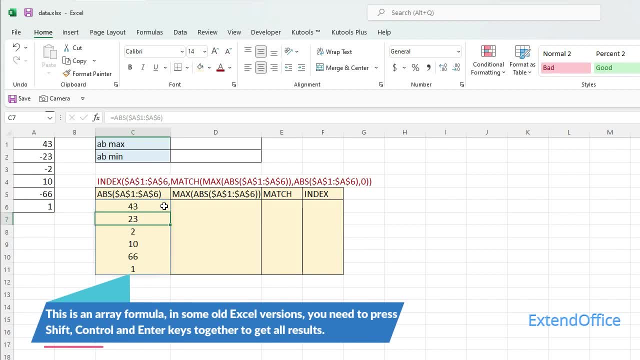 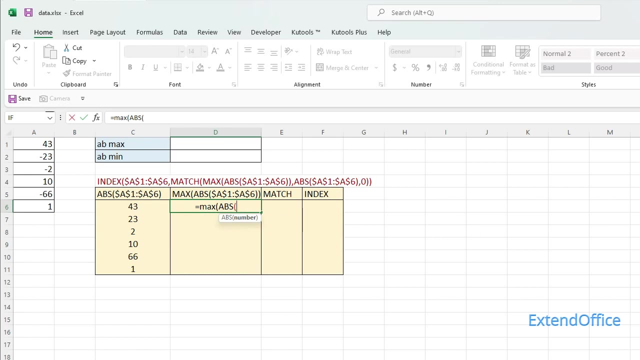 In this example, I need to press shift and enter keys together to get all the results. This is an array formula. Combine MAX and ABS functions to get the maximum absolute value in the range. 66 is the maximum absolute value in the range. 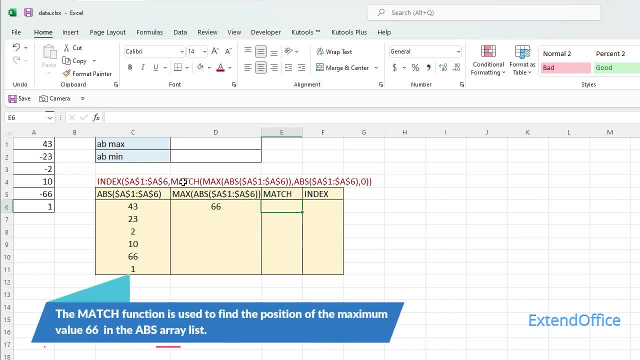 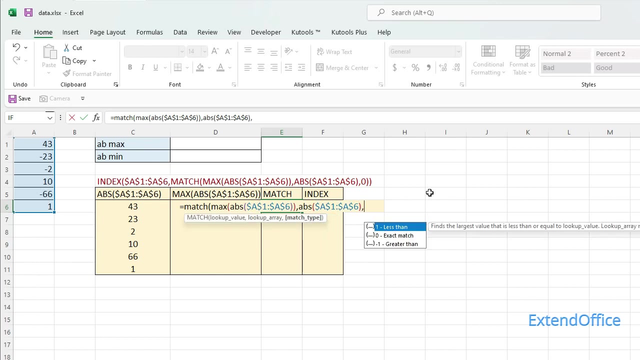 The MATCH function is used to find the position of the maximum value 66 in the ABS array list. The MATCH function is used to find the position of the maximum absolute value 66 in the ABS array list. The MATCH function is used to find the position of the maximum absolute value 66 in the ABS array list. 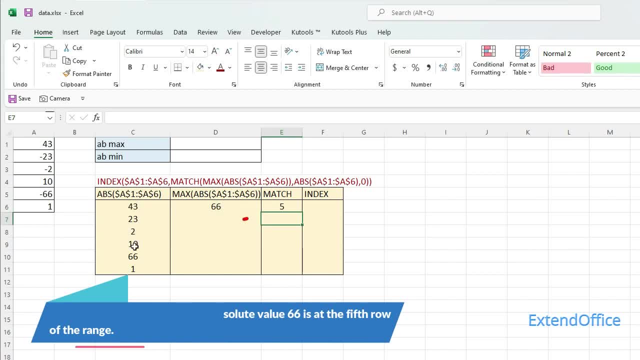 The maximum absolute value 66 is at the 5th row of the range. Finally, INDEX function is used to return the value that at the 5th row of the range. Finally, INDEX function is used to return the value that at the 5th row of the range. 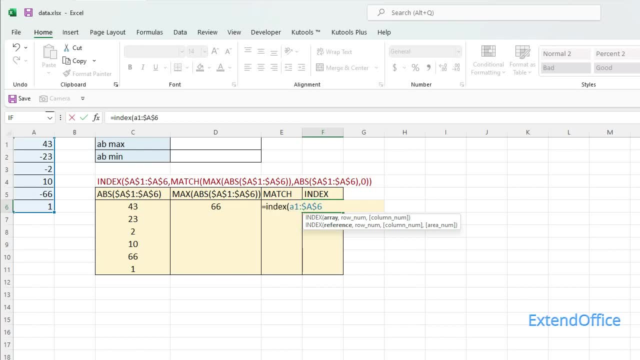 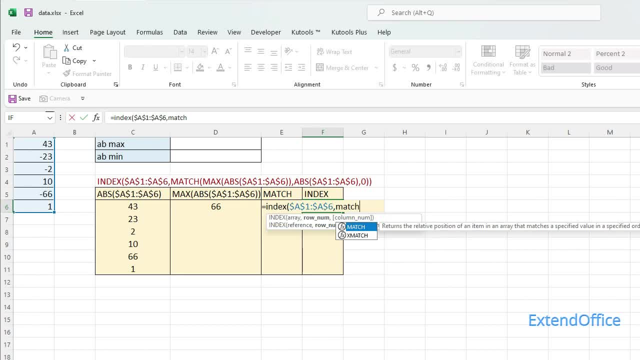 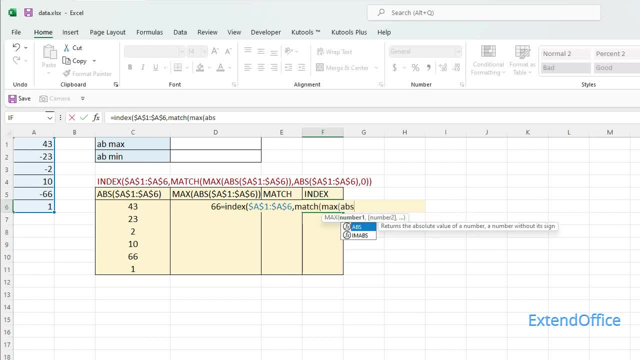 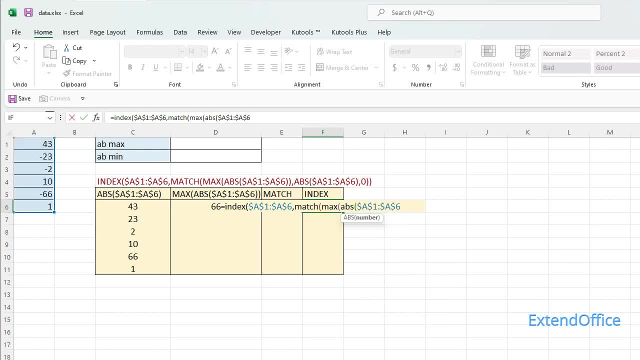 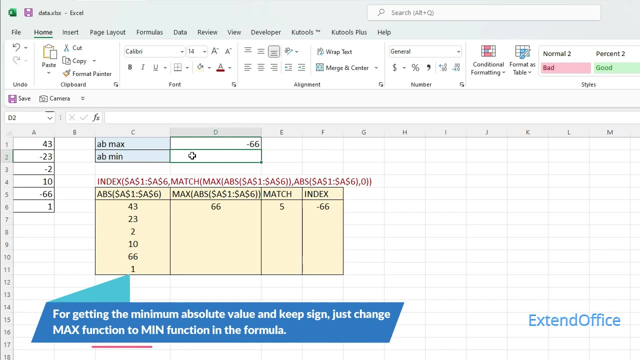 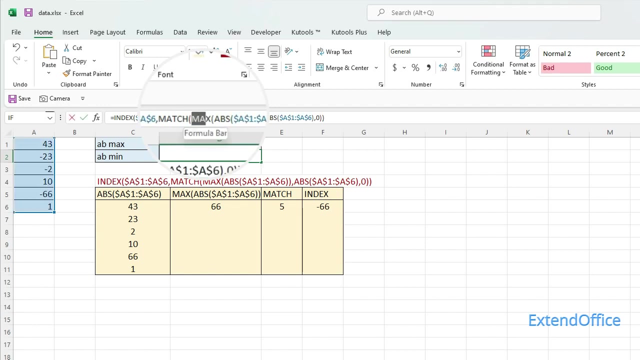 Now the maximum absolute value and keep its sign is returned. For getting the minimum absolute value and keep sign, just change max function to mean function in the formula. Notice that in old Excel versions press shift control and enter key to get the correct result.